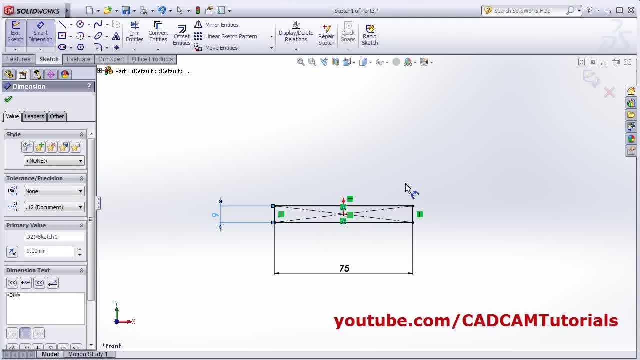 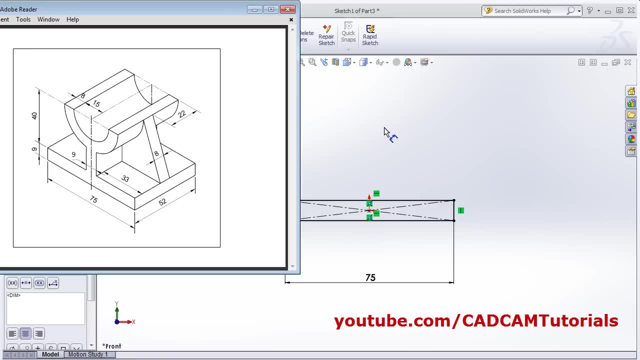 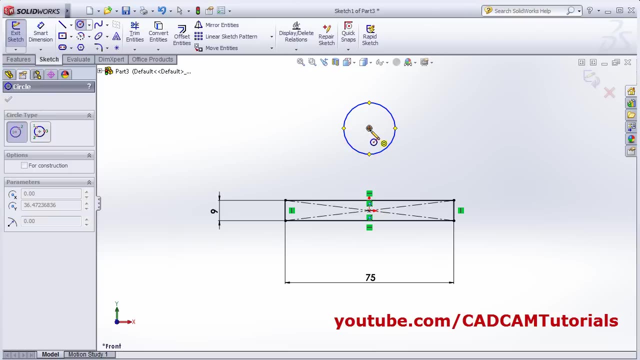 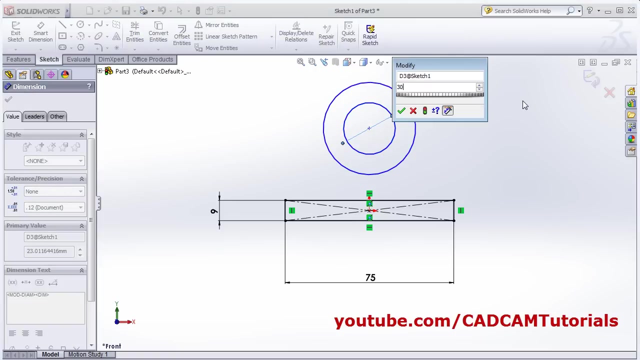 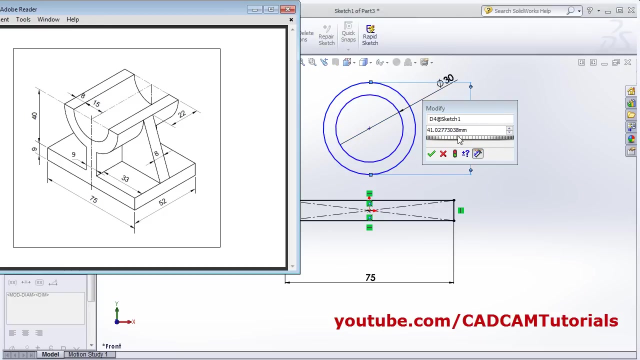 And width is 9.. Then next will be these two circles of 15 and 23 radius. Click on circle. Track the point. Create two circles. Smart dimension: internal is 15,, that is 30 diameter, And external is 15 plus 8, 23.. That is 46.. 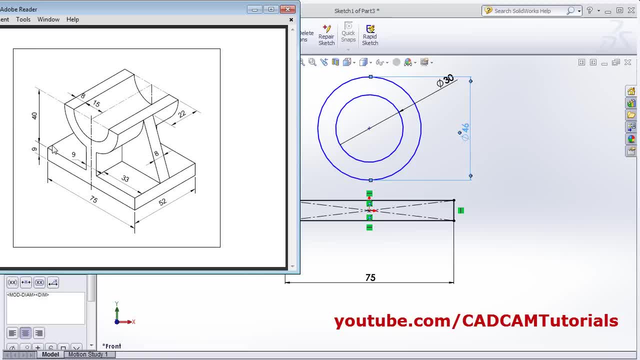 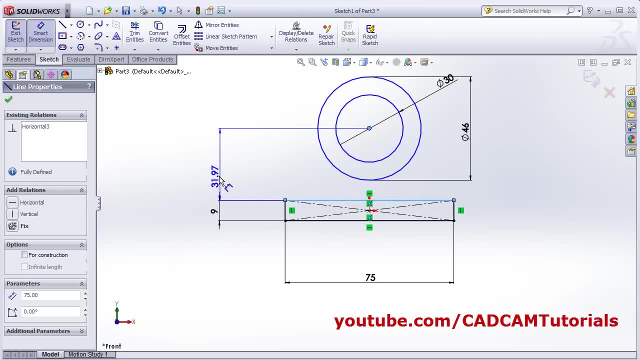 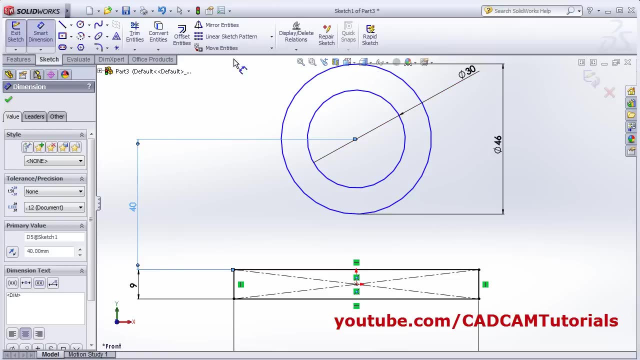 Then the height of circle from this top line is 40. Given, smart dimension is already on, Click on this center point and this horizontal line. Give the gap of 40. Then we don't need above circles, Create one line from quadrant to quadrant. 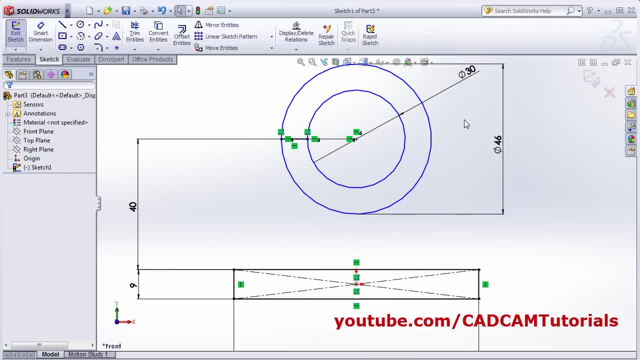 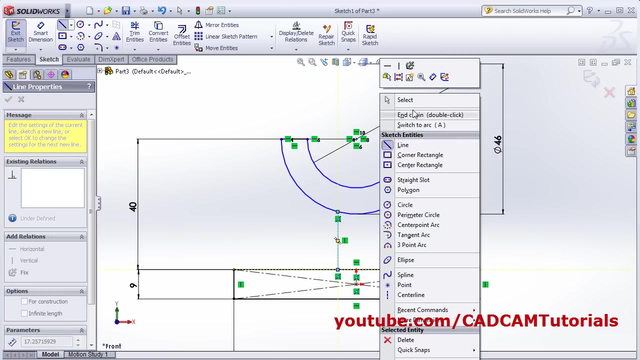 select: right click select. right click line from this quadrant to this quadrant. right click, select. then trim unwanted object. click on trim to closest and remove the unwanted object. right click, select. in here vertical lines are required. click on line. create one vertical line from here to here. right click, select. then this line will be symmetric around. 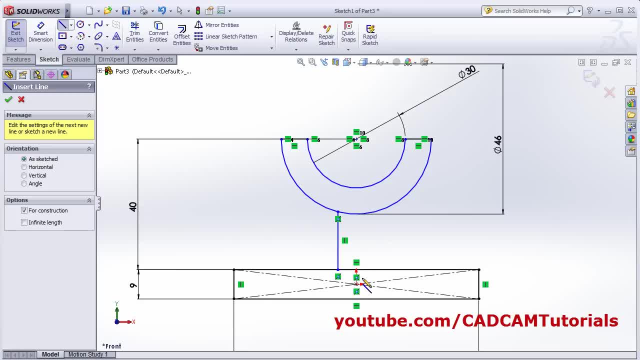 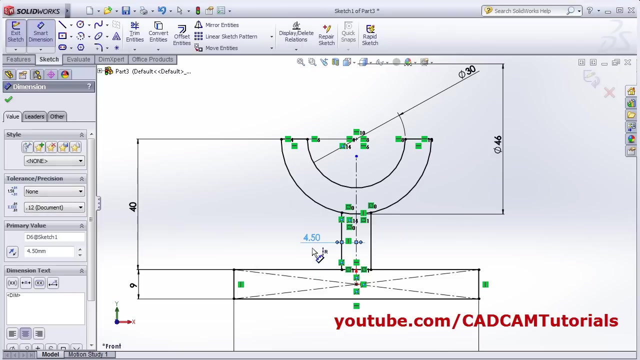 vertical axis. create one center line. right click, select. then make it symmetric. select this line, mirror entities, click on mirror mirror entities and mirror axis will be this line. done then give the gap will be 4.5, you smart dimension- from this axis to this line 4.5. then again trim. 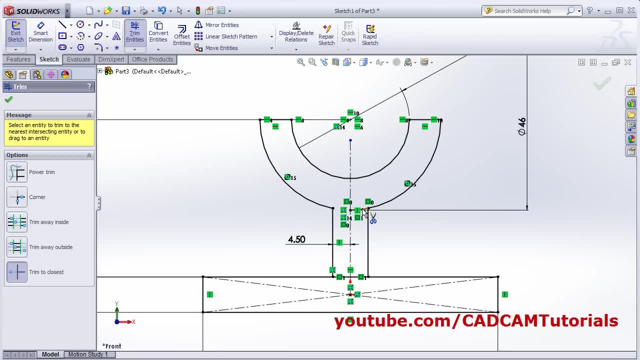 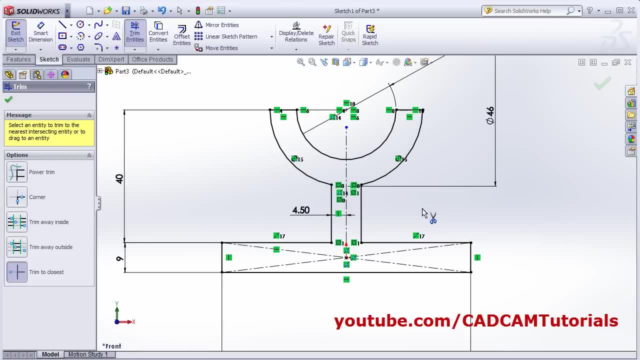 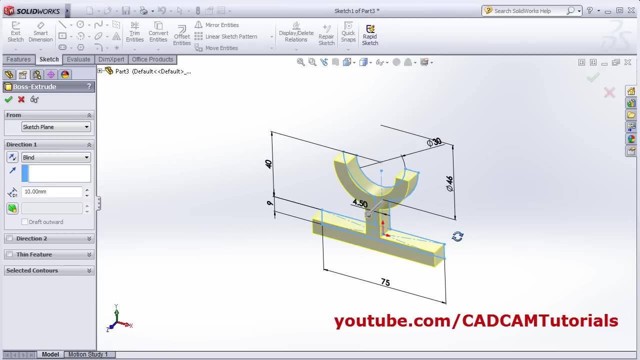 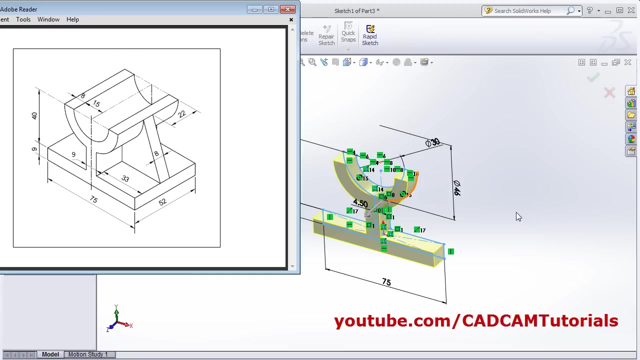 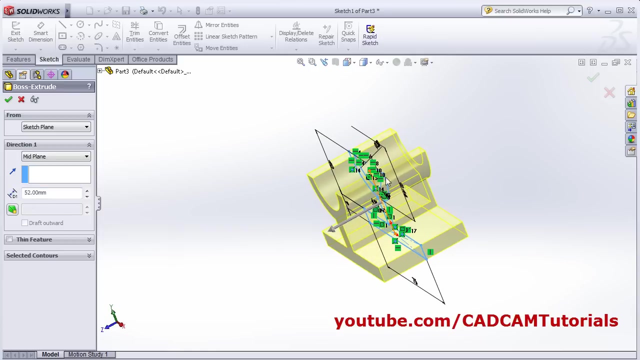 the unwanted, trim entities and make a close object. okay then. okay, back you, then I want to extrude it around center, on both sides. so therefore I will take this option midplane and give the total width of 52. I am taking this midplane so that 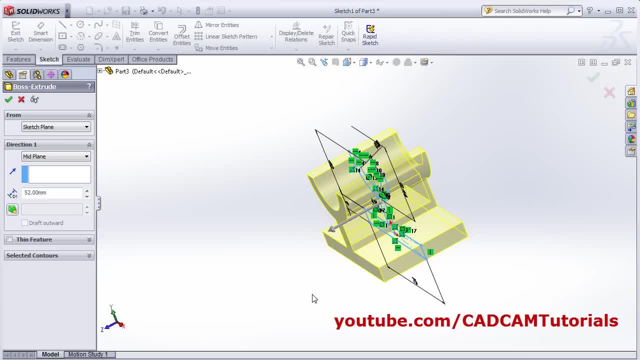 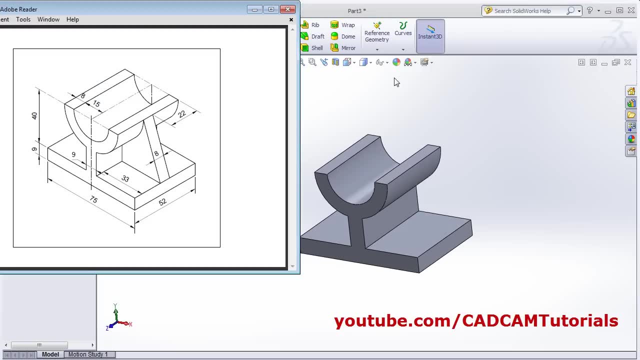 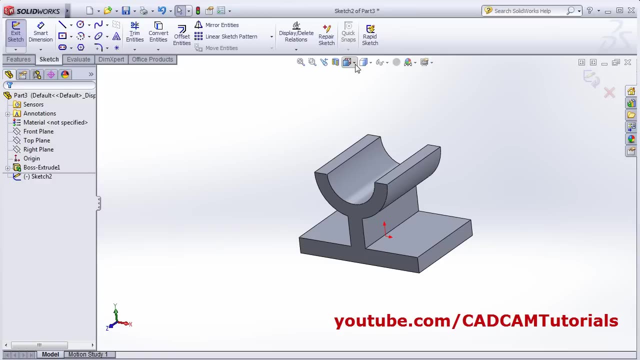 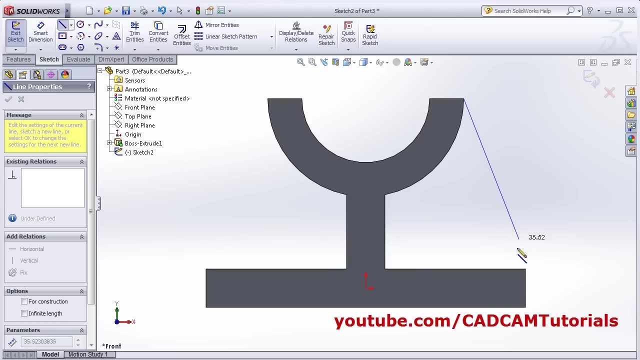 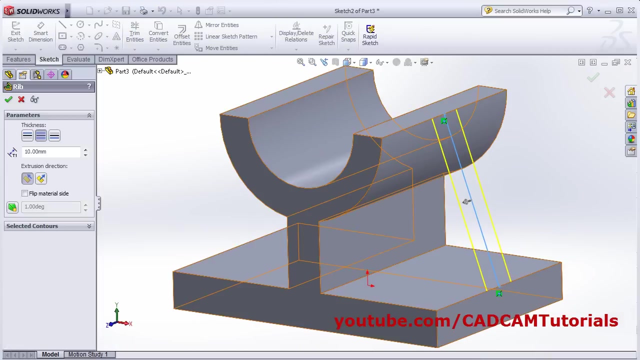 we can create this reap on the center plane and click on ok. the next will be be to create this rib. click on this rib and select this front plane and click on normal normal to create one line from this end point to this end point, right click, select and back, then give the thickness of 8 and it is around both. 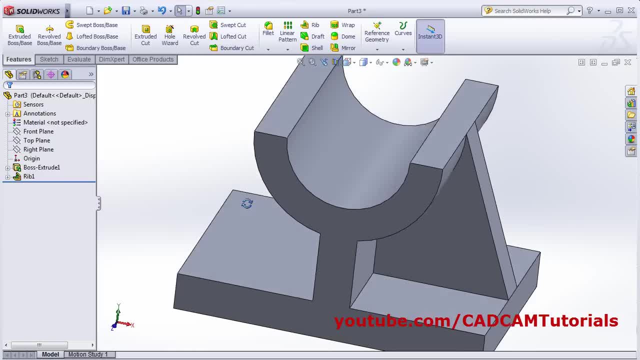 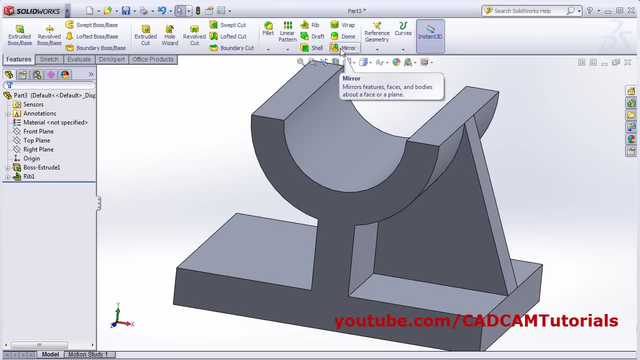 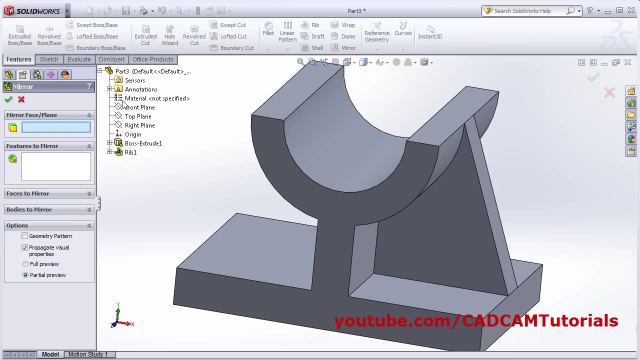 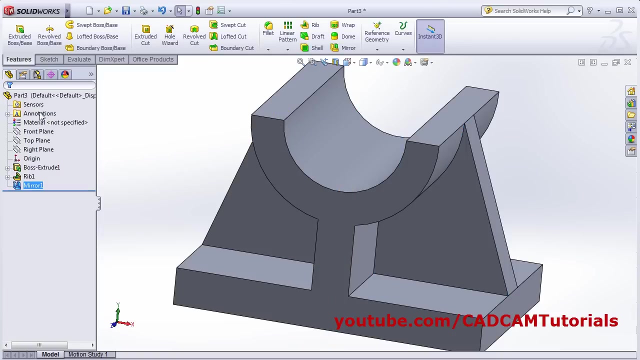 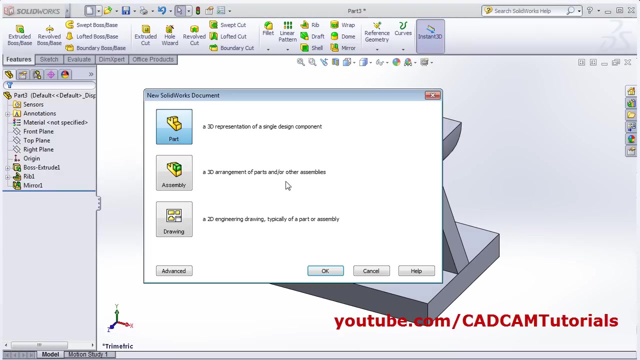 sides. then okay, then same rib I want on the opposite side also. so select the mirror, click on mirror, then select mirror plane, so mirror plane will be at the center here. and select this right plane, then features to mirror, select this feature and click on ok and isometric view. this object is ready. again click on new okay. 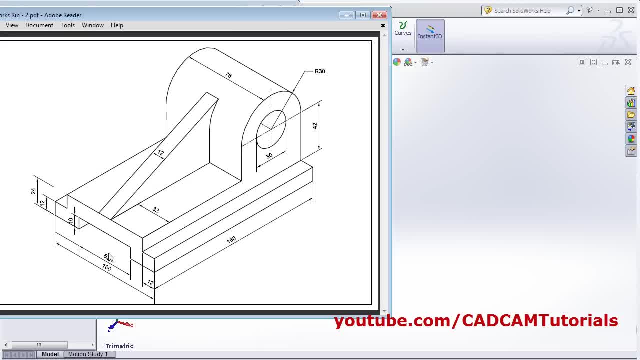 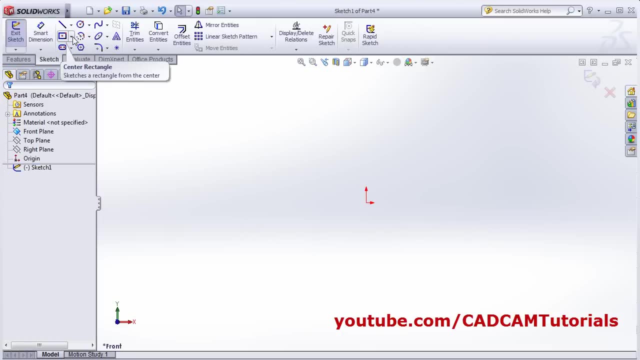 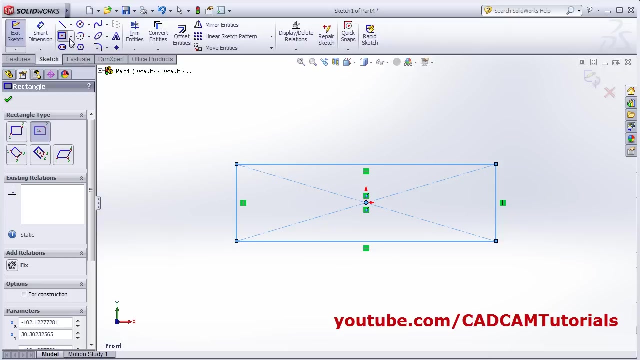 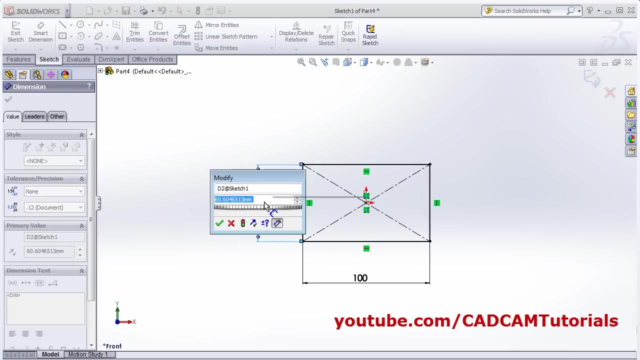 then next object is this one. in this object, at first we will create this rectangle of 100 by 24 on vertical plane. click on extruded boss base, select this front plane and select rectangle center, rectangle smart dimension. give the length of 100 and width of 24, then back and give the total. 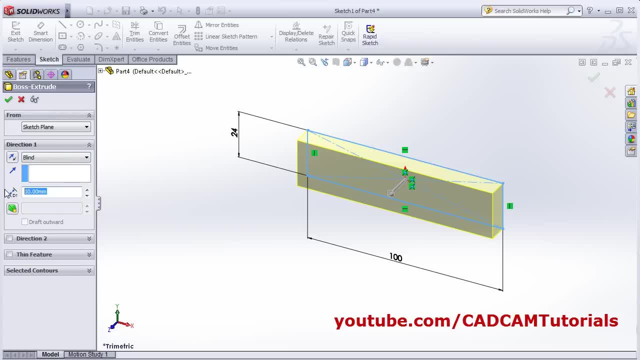 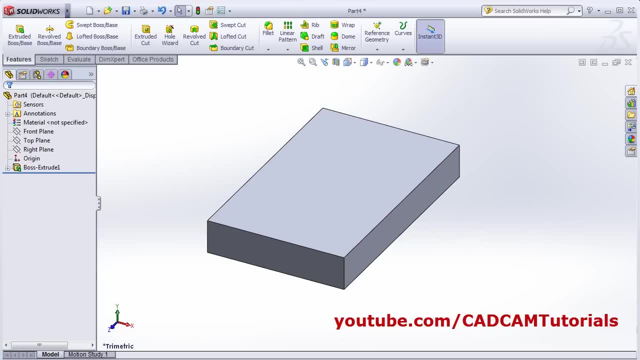 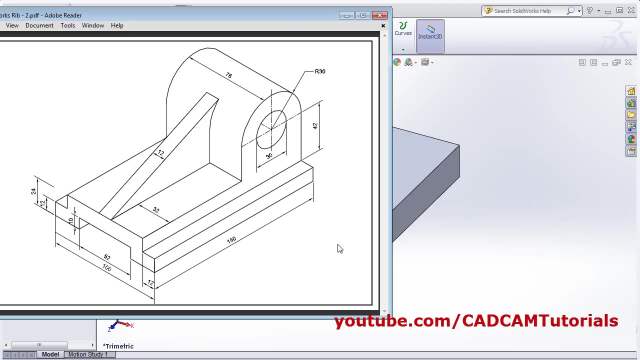 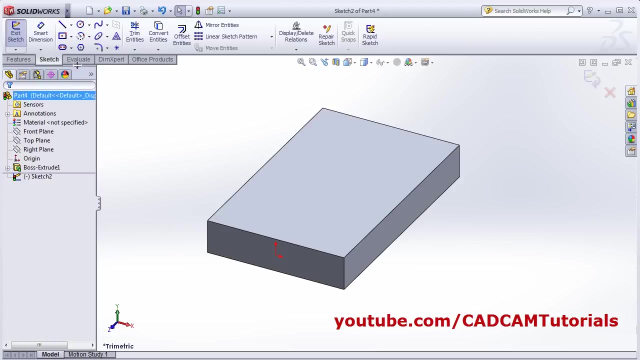 length of 160 O backward. click next will be this Dean: okay, then 来春. or 52 by 10, the gap is 24. this line length is 24. click on extruded cut, select this surface, then create one rectangle, two point rectanglelands. from here to this vertical line is 24, then internal length is 52 and 10, so this height. 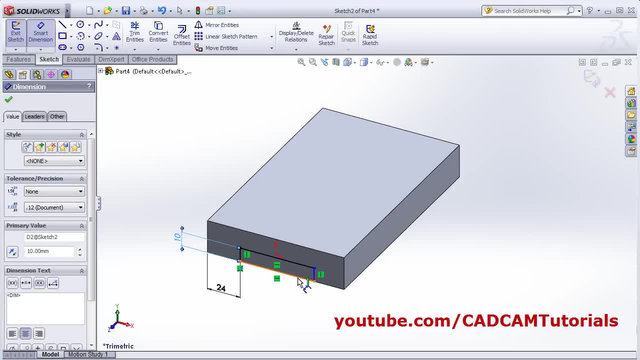 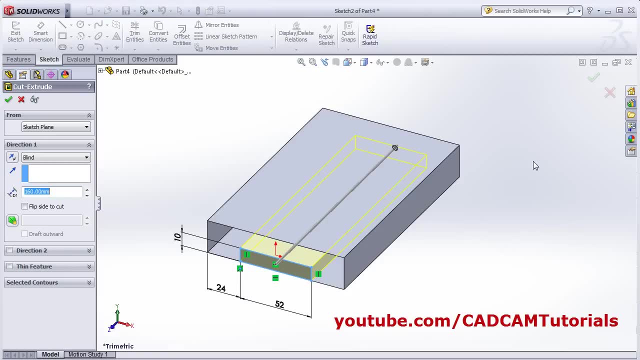 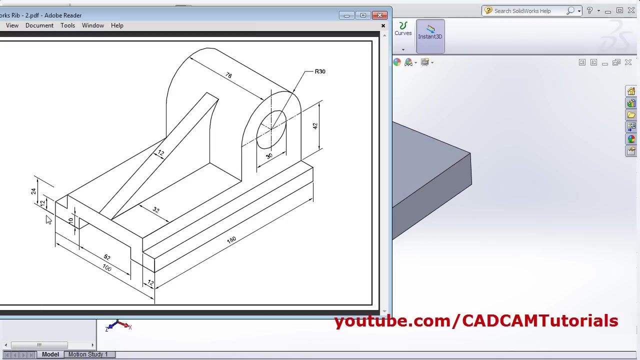 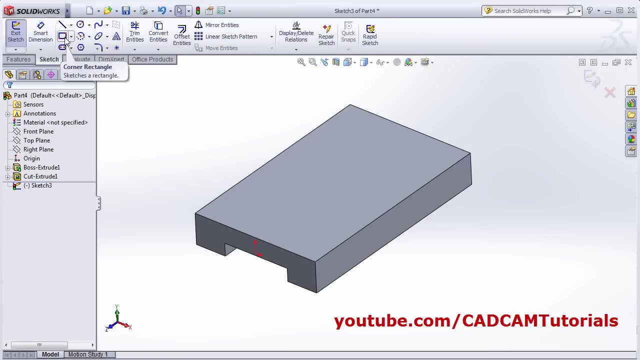 is 10 and this length is 52. then back now i want it through, so click on through. all okay, so it is cut throughout. then next will be this cut, small cut of 12 by 12- i'm again extruded. cut, select the surface, create one rectangle, corner, rectangle from this corner. 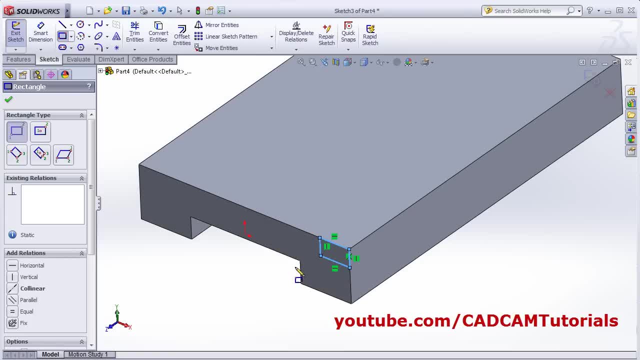 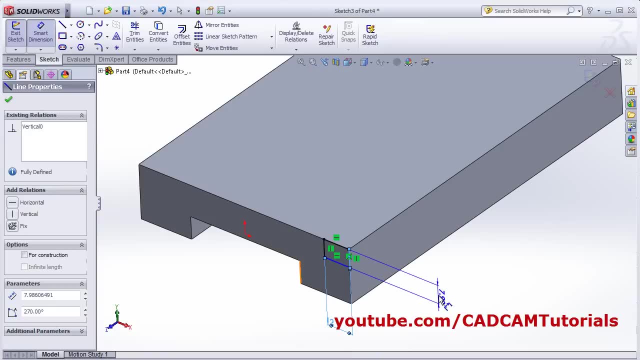 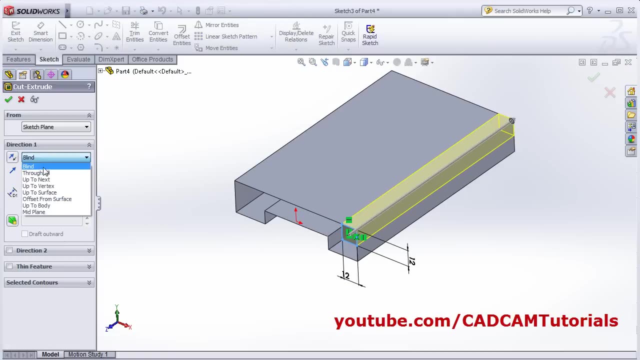 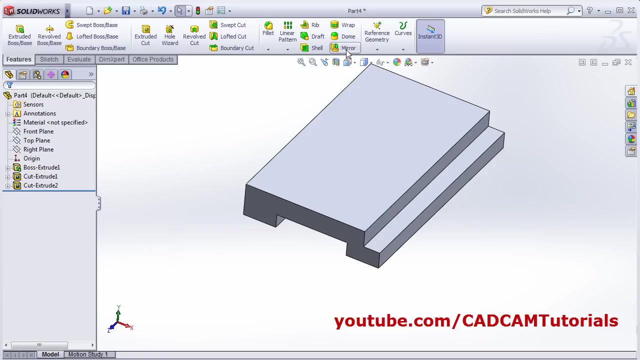 to inside. give the parameter smart dimension. this is 12 and this is also 12.. okay, then back again through all. okay, the same i want on the opposite, so we can mirror it. click on mirror select. the plane plane will be the center plane. click on this plus and. 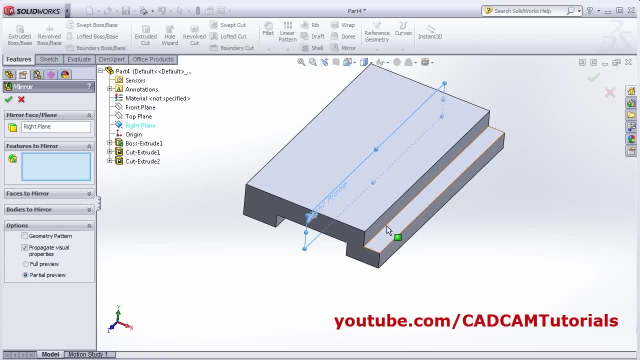 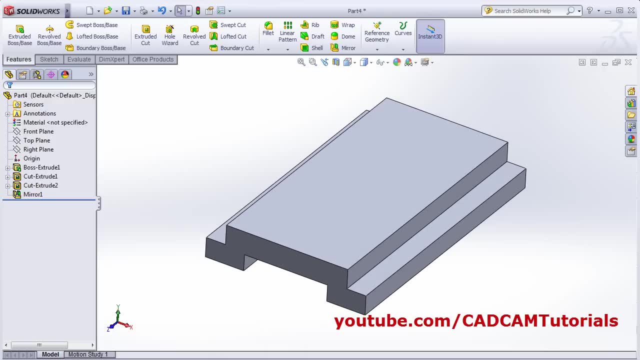 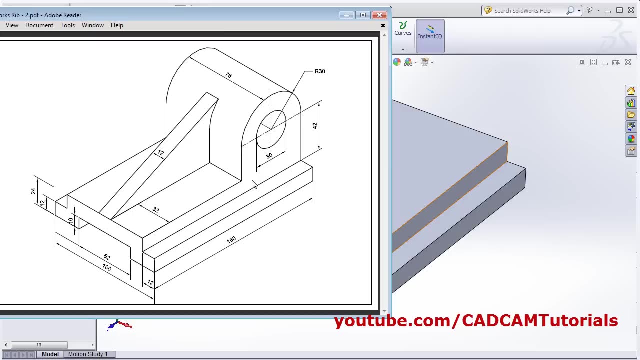 click on this right plane feature to mirror. is this feature okay? zoom fit okay. so the next portion will be this portion. for this portion, we will create one rectangle of 60 by 76 and we will extrude by now this 12. we are not considering that means 30 plus. 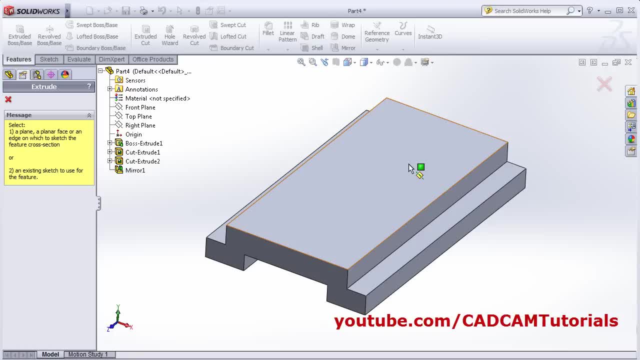 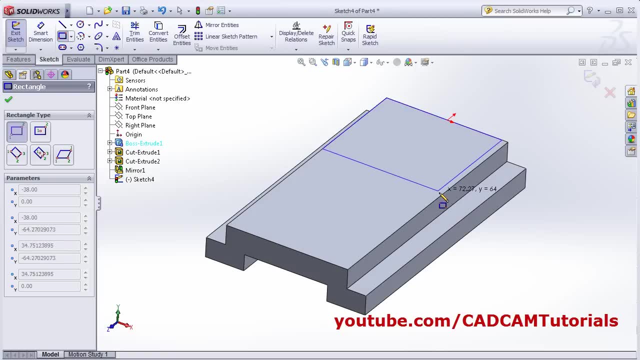 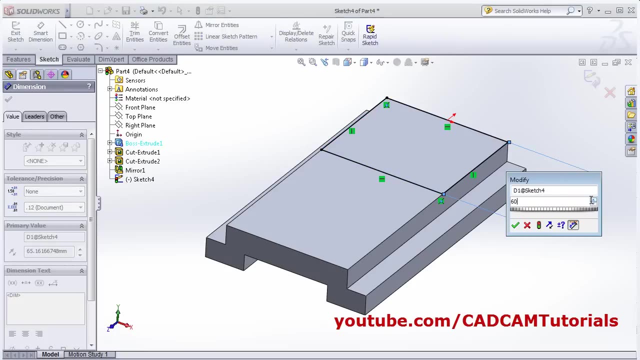 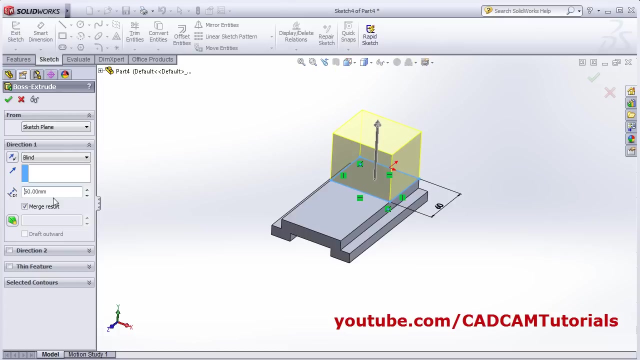 30, 60.. click on extrude bosbys. select this surface. then select this corner rectangle from this corner to this edge. then select the corner rectangle from this corner to this edge. then smart dimension. length of this line is 60. then back, the height is also 60, okay. 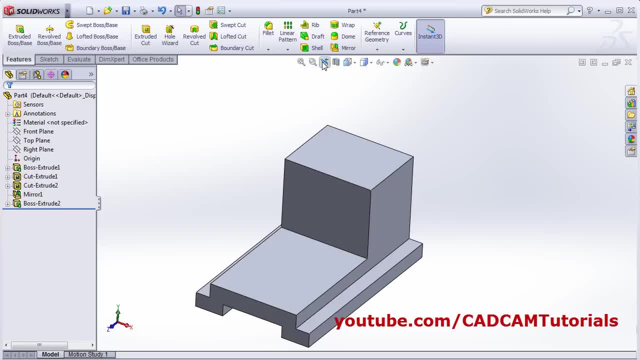 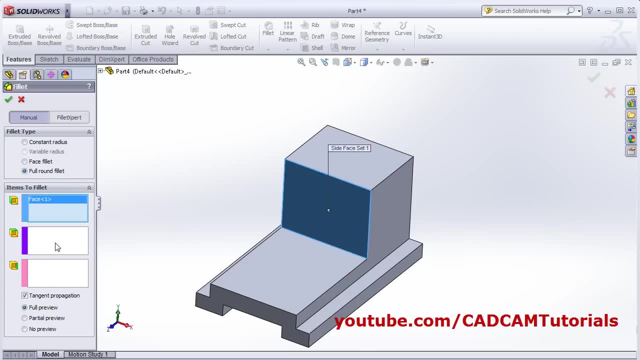 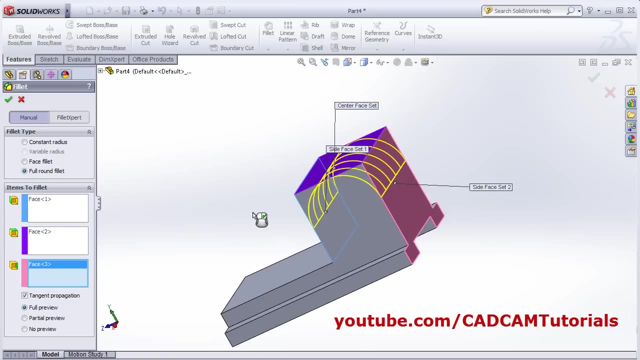 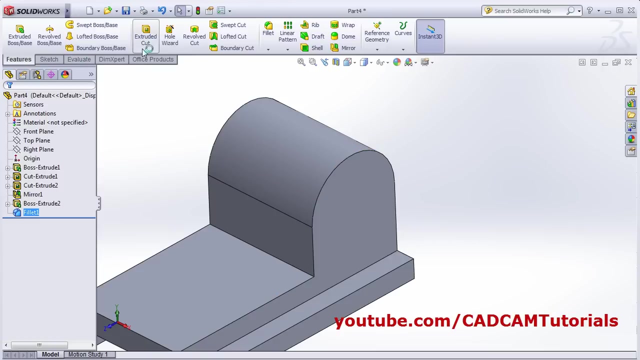 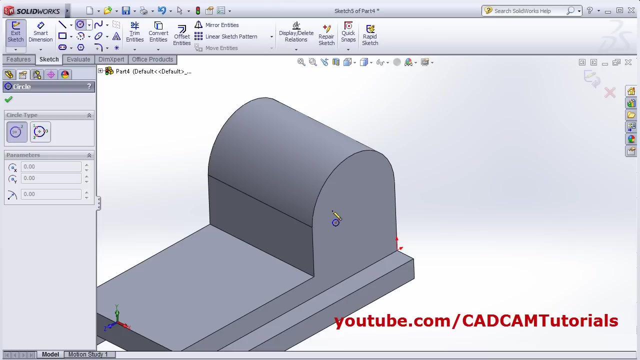 then we want a circle here for that. click on fillet, then select foreground fillet, select this surface and send. select this surface. click here and select this surface, then okay, you know one hole is needed here. click on extruded cut. select this surface. click on circle: create circle at the center.